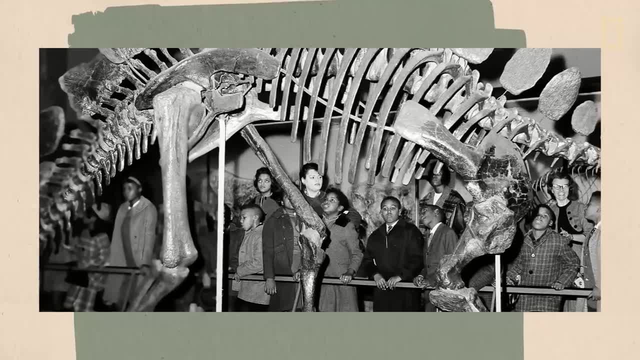 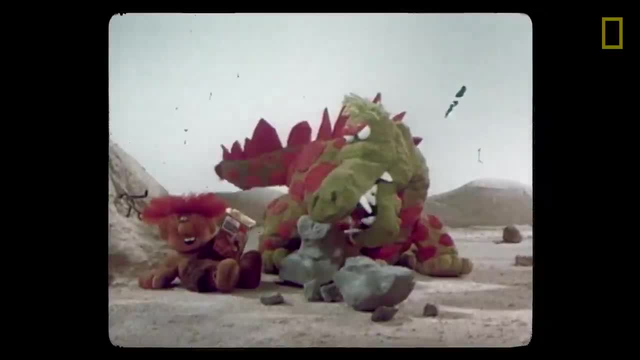 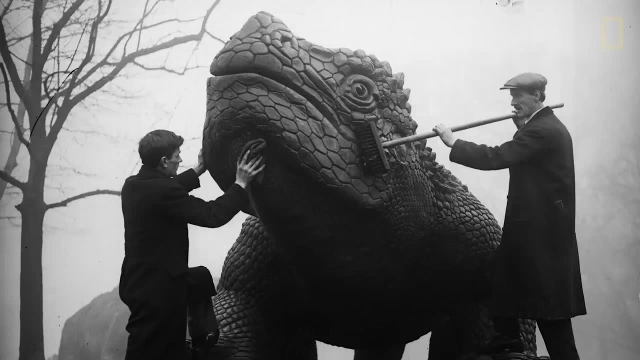 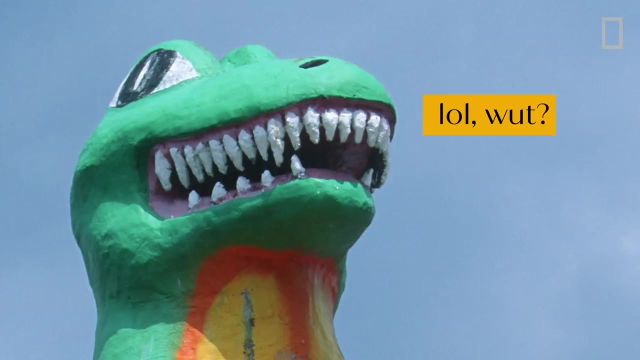 was high, so a view into this prehistoric world came from a different perspective. Art Creativity brought dinosaurs to the cultural forefront. While these drawings, paintings and sculptures were initially based on scientific discoveries, let's just say that didn't last. 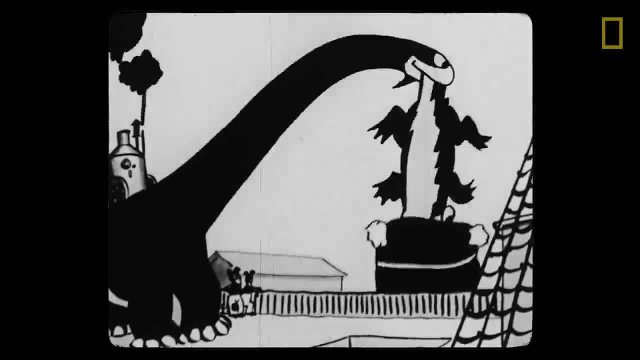 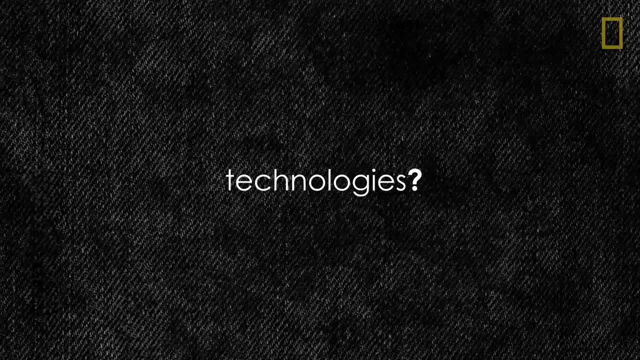 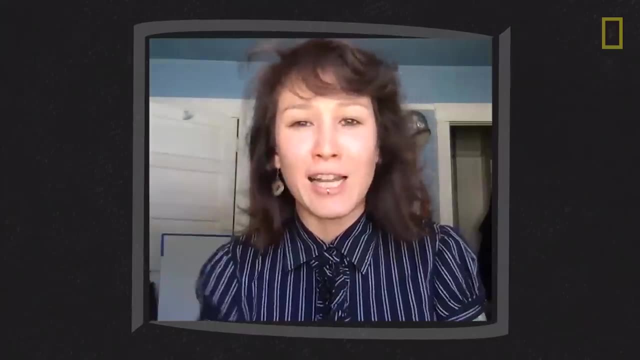 Our imaginations might have gotten a head start, but technology it's catching up. Paleontology has been undergoing this massive revolution. One of those technologies, CT scanning, giving paleontologists a new look at dinosaurs. You can look at the brain size. 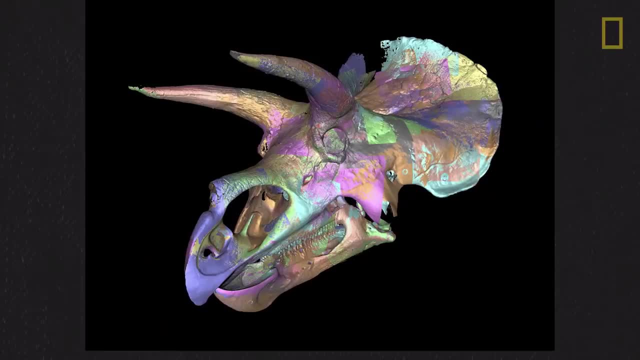 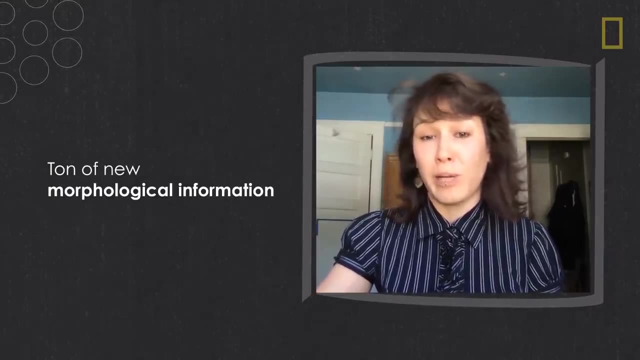 You can look at the different parts of the brain, because basically, the bones that demarcate the brain cavity are very good proxy for what the brain actually looked like. So there's a ton of new morphological information that we can get through these high resolution. 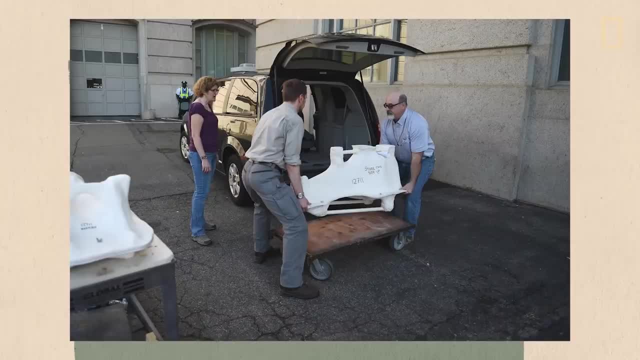 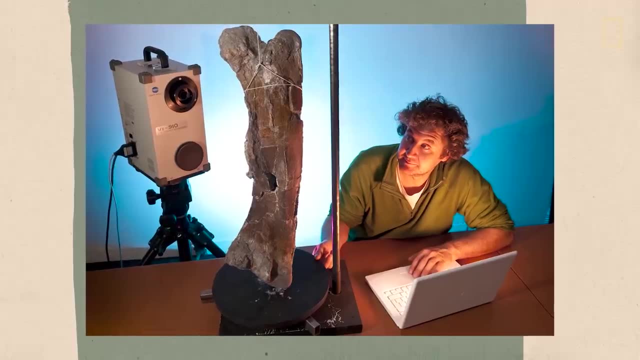 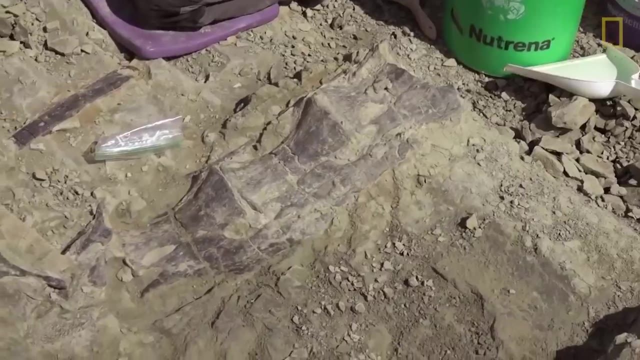 imaging techniques that are fairly new. This in-depth view has been a game changer in the field, But one classical aspect of paleontology has also experienced a renaissance: Finding fossils In the US or in Europe- that's where paleontology first grew as a science. 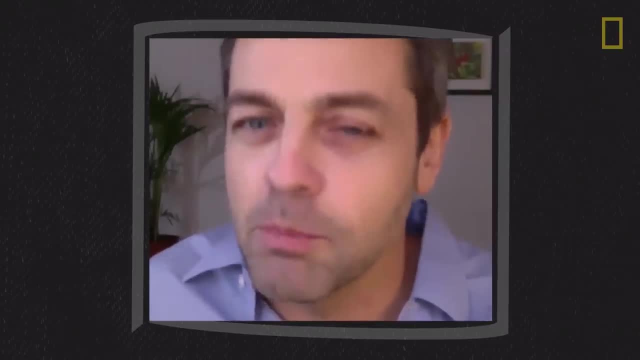 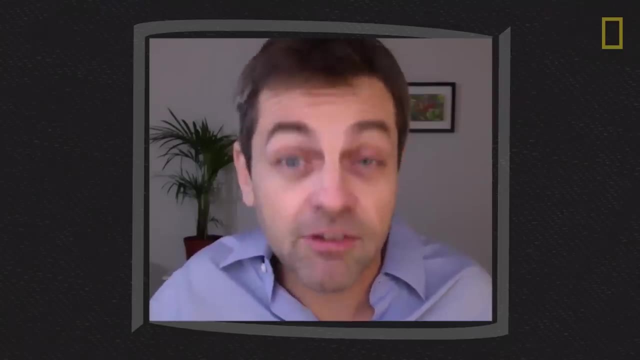 But other continents. they have not been explored as much. There are so many expeditions being conducted right now. Many, many new dinosaur species are coming from this place. For example, Diego's team in Patagonia discovering the Patagotitan Majorum. 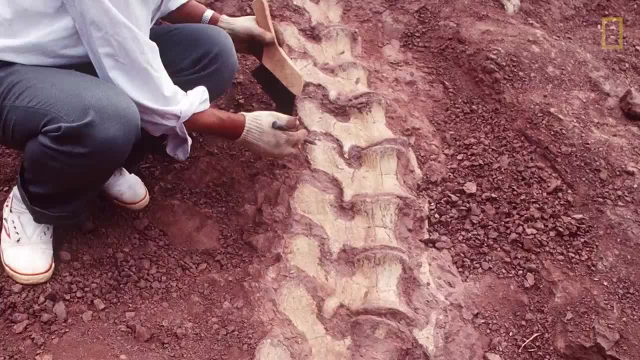 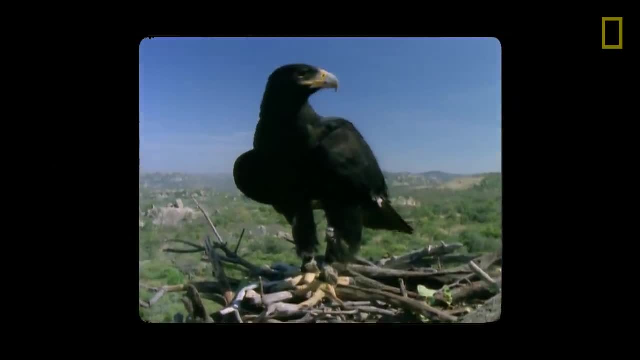 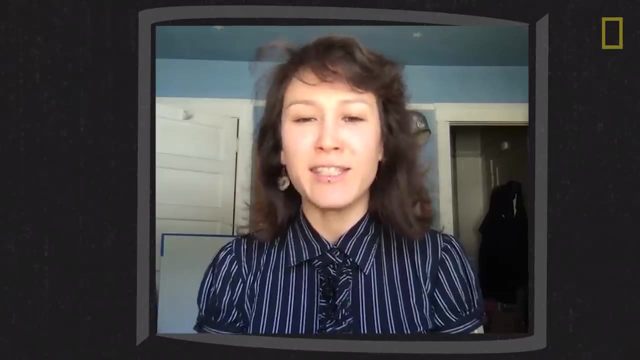 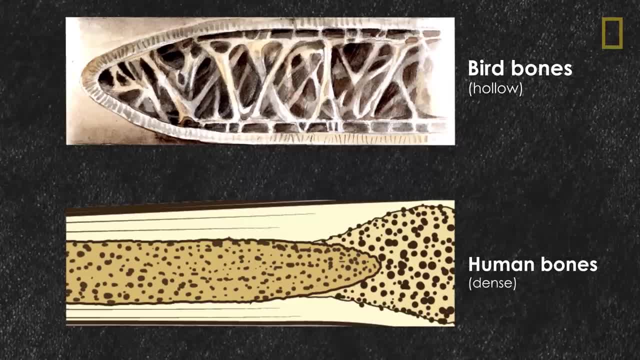 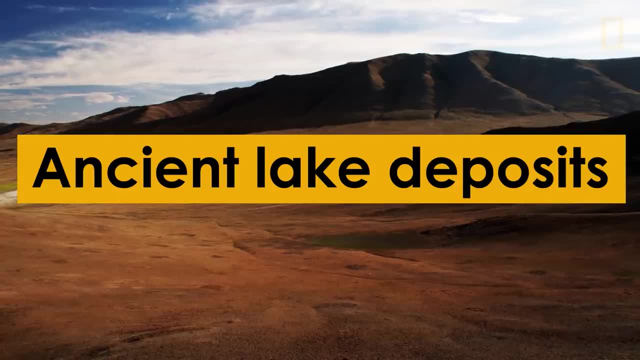 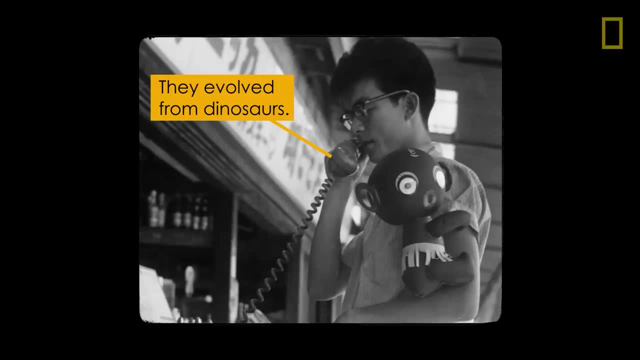 The other thing is that birds have hollow bones. They get crushed easily, they get destroyed and they just don't survive. So all these fossil birds all come from ancient lake deposits. The perfect environment to preserve these very delicate fossils- Birds evolving from dinosaurs- is not a new idea. 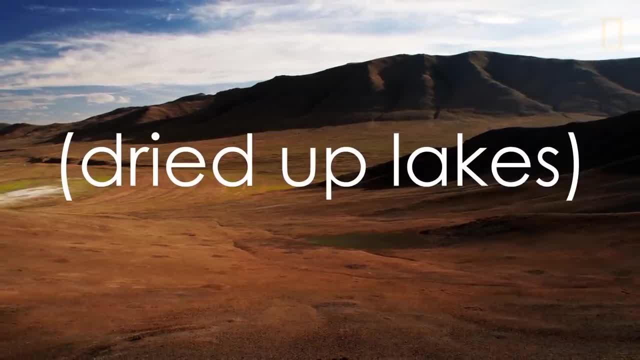 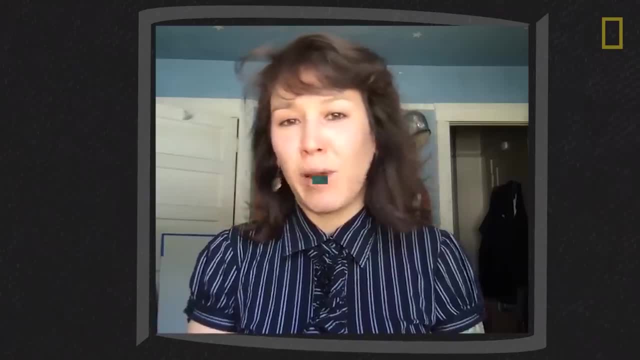 but it's the access to these ancient lake deposits that's finally providing the necessary evidence. The notion that birds are living dinosaurs actually dates back to like the second half of the 19th century, A guy named Thomas Huxley. based on his observations, 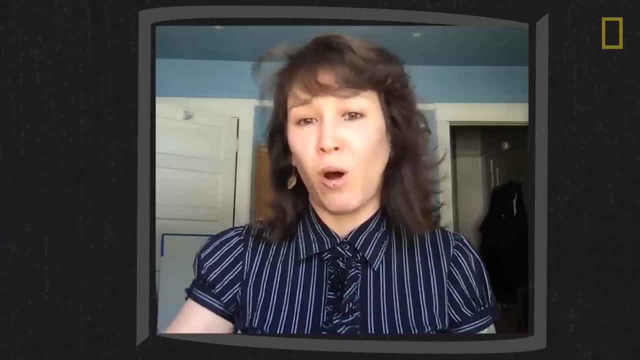 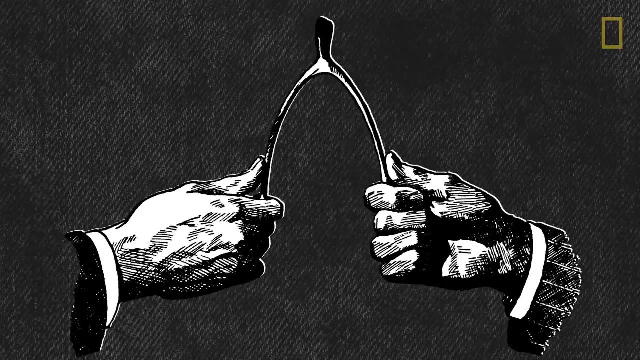 he came up with a hypothesis that birds descended from small bipedal dinosaurs. But other scientists opposed this idea because they said: well, you know, all birds have a wishbone, right? This is not known in any dinosaurs, so birds can't be living dinosaurs. 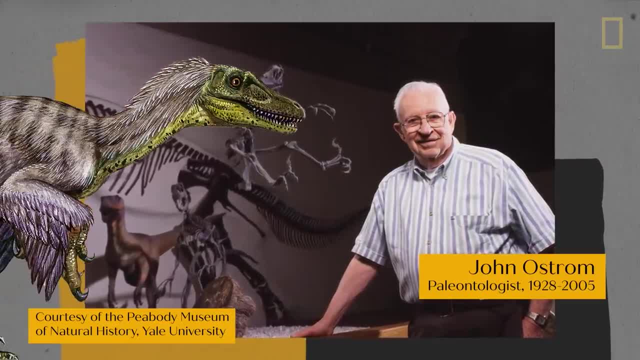 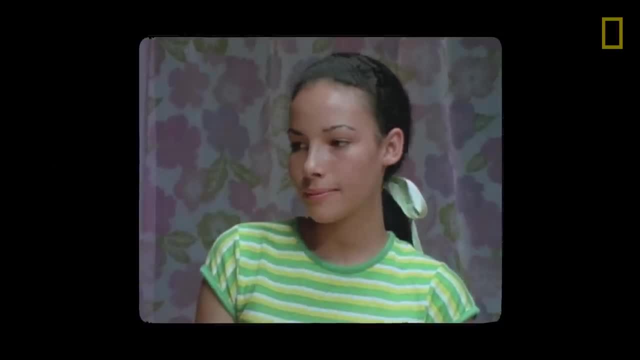 Next up John Ostrom, who analyzed theropod dinosaurs and also hypothesized that birds were living dinosaurs. But again people kind of rejected this hypothesis At the time. their new reason was velociraptors that were supposed to be closely related to birds. 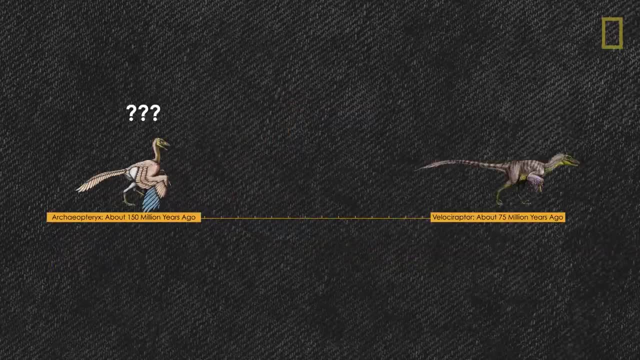 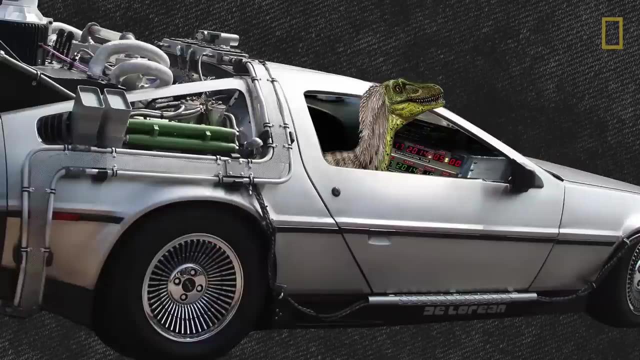 were much younger in the fossil record than Archaeopteryx, the oldest bird. So they were like: how could Archaeopteryx have descended from taxa that don't appear in the fossil record until like 70 million years later? right Inconclusive evidence persisted until 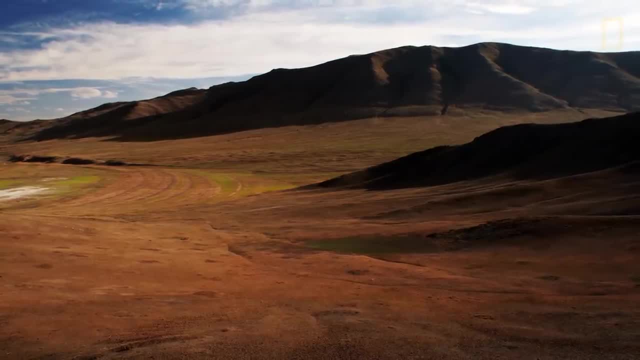 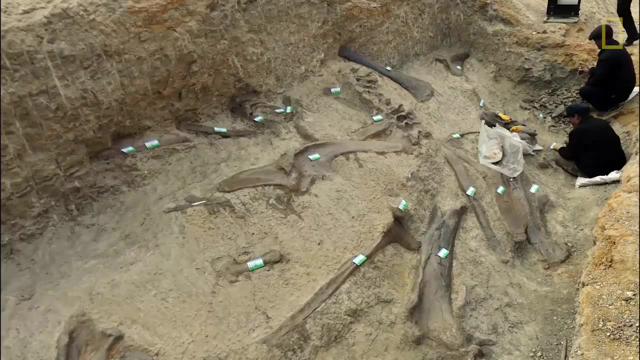 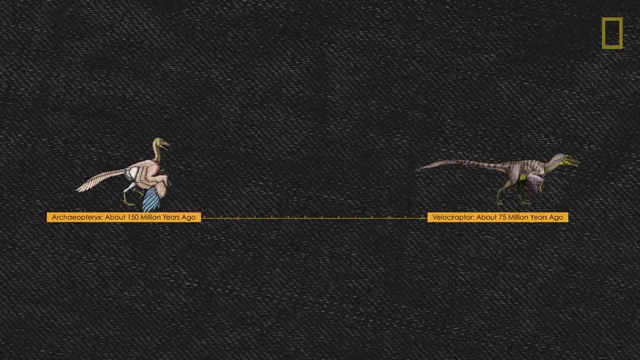 well, that's what brings us back to these ancient lake deposits. So in 1996, you find the first feathered dinosaur in China. So then an enormous amount of field work started to happen, and this produced these thousands of specimens. Paleontologists then discovered an area. 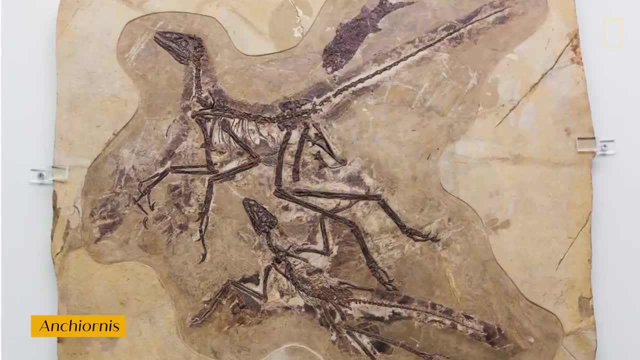 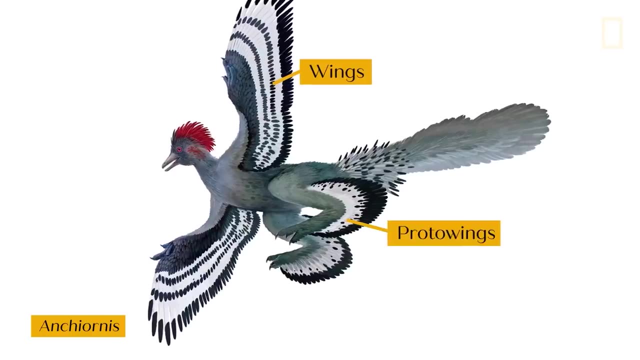 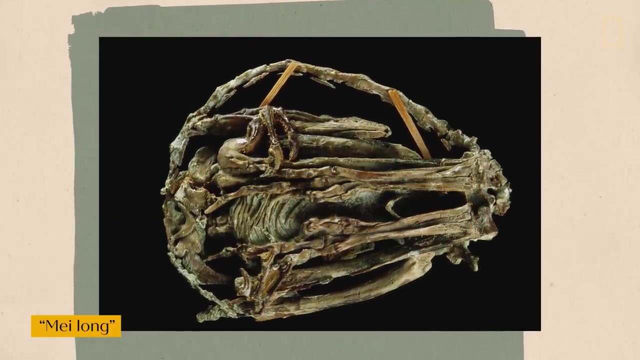 where fossils predate Archaeopteryx, And within this area they found small feathered dinosaurs with bird-like traits, including wings here and here, making his theory much stronger. Also, There was a little troodontid dinosaur named Meilong. 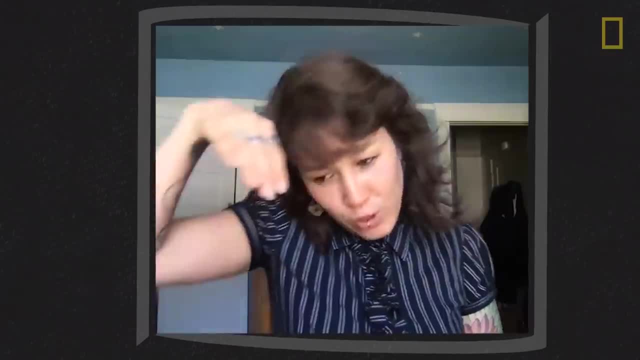 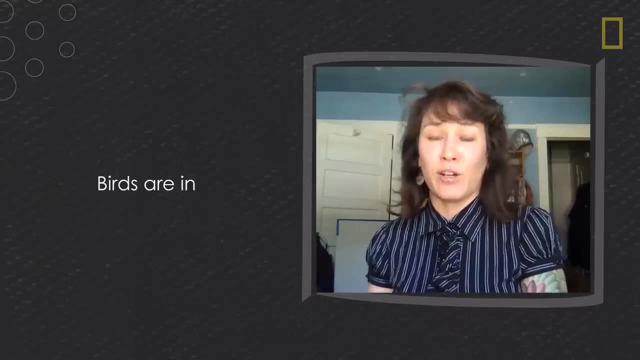 that was discovered and it's really tiny. It's like this big- and it's preserved with its head underneath its wings, sleeping the same way modern ducks do. So that's behavioral evidence that birds are in fact living dinosaurs. Today, substantial evidence points to birds 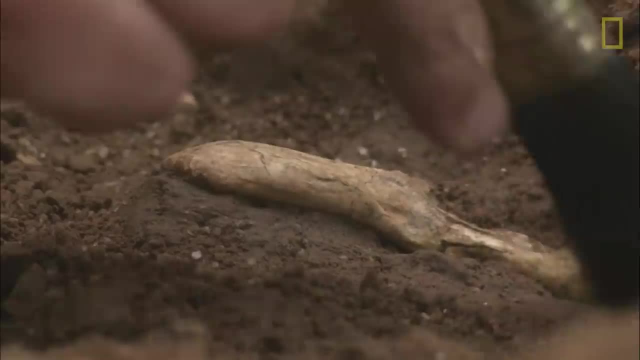 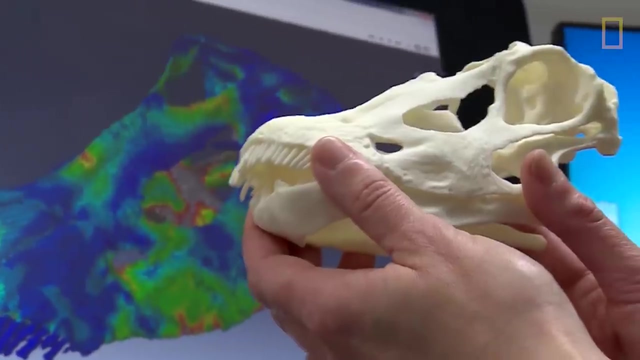 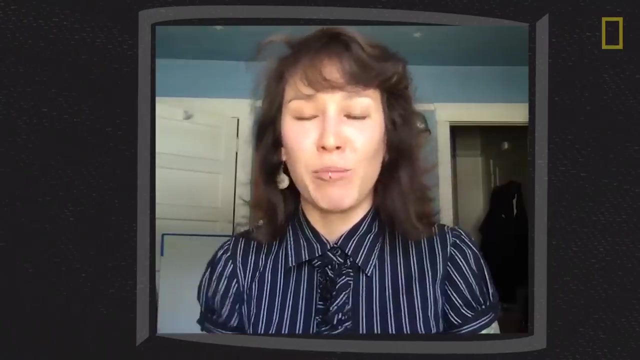 evolving from dinosaurs, specifically theropods, and showcases the progression of paleontology. But the discoveries don't stop here. There are still new things out there that, once they are discovered, are going to shake up everything we think we know. New data will cause us to adjust to our existing hypotheses.